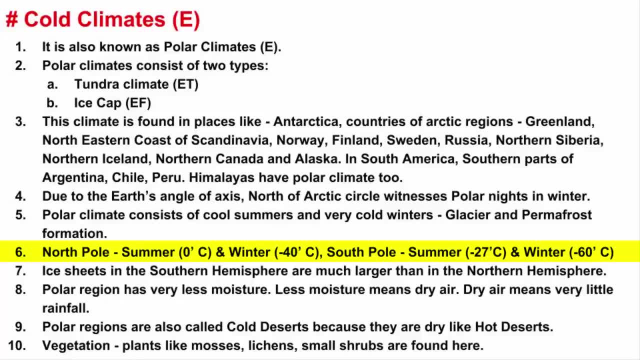 And if you look at the south pole has an average temperature of minus 27°C during the summer and minus 60°C during the winter. These places are so cold. when the snow falls it does not melt. it gradually accumulates over hundreds and thousands of years to make a 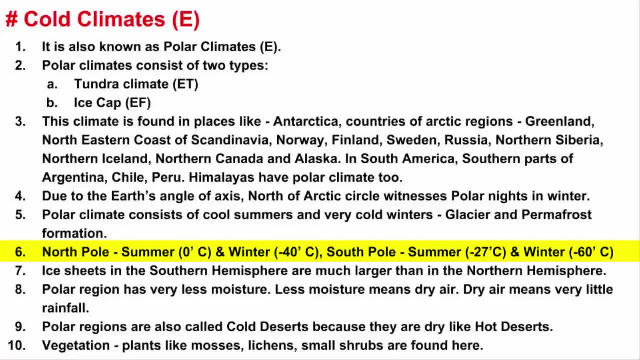 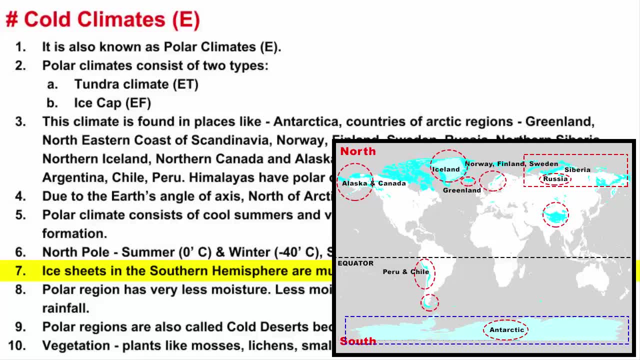 thick ice sheet called permafrost. The ice sheets in the southern hemisphere are much larger than in the northern hemisphere, larger than in the northern hemisphere, covering the entire continent of Antarctica. and if you look at the seven continents of the world in order of their size, Antarctica is at fifth position. 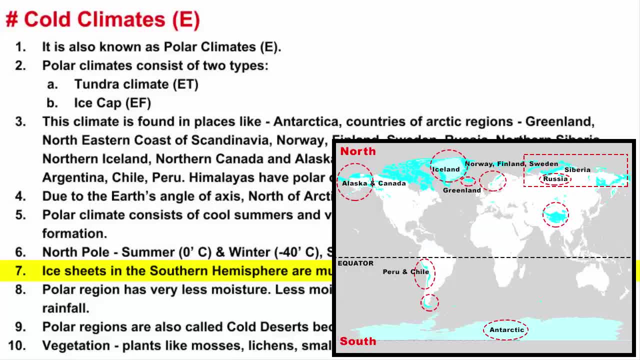 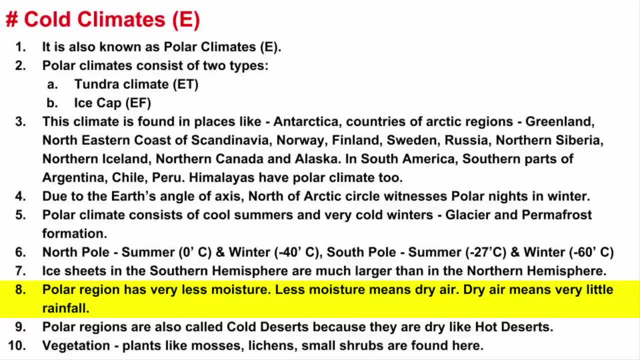 therefore, the southern hemisphere has more ice sheet compared to northern hemisphere, since the air in polar region is so cold that it contains very little moisture. again, it is because of the sun rays, because half the year the sun does not rise above the horizon, and since there is very little moisture, the air is dry, and dry air means that there is very little snowfall. 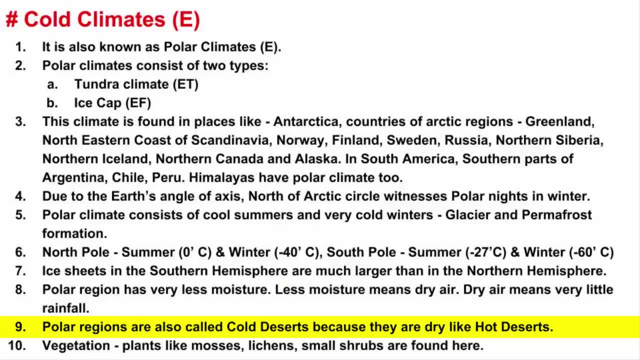 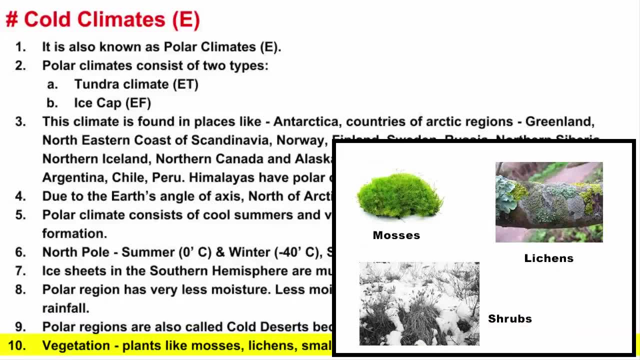 polar climates can be dry as the hot desert. that's why these regions are also called cold deserts. coming to the vegetation part, the only plants that can survive the harsh winters and wet summers are small ground hugging plants like mosses, lichens and small shrubs.